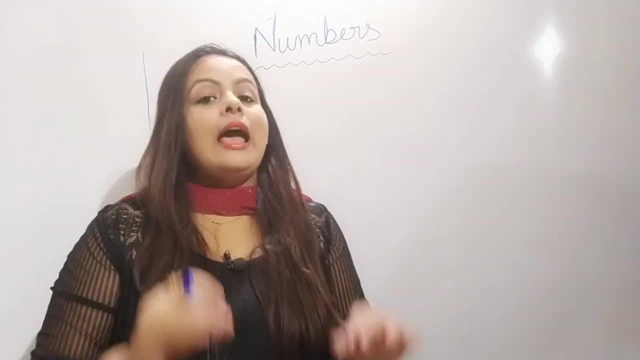 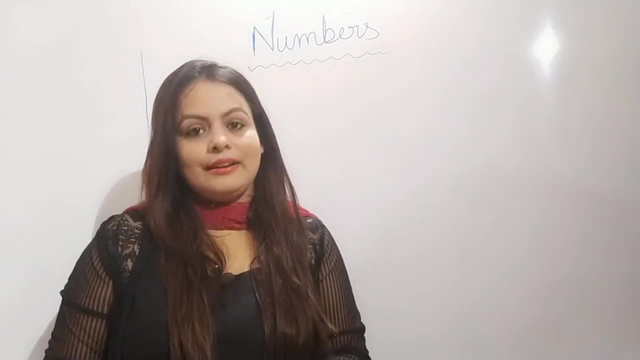 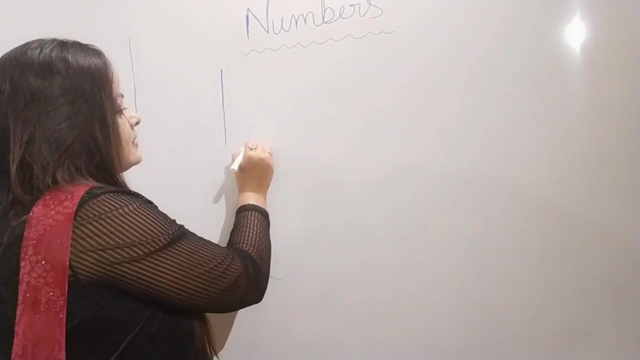 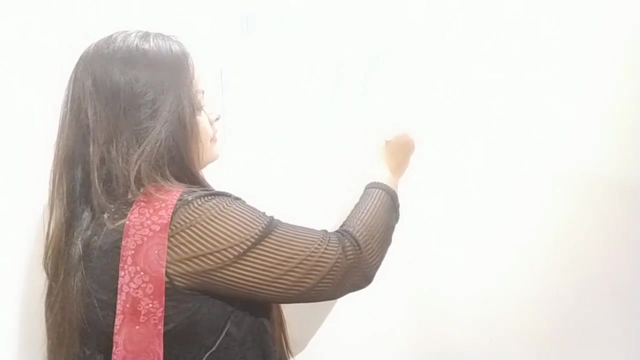 few curves so that your little one can understand and it will help your little one to write the numbers okay. with the help of the strokes and curves they can easily write the numbers okay. so now let's start standing line, slipping line, slanting line c, curve half a circle and 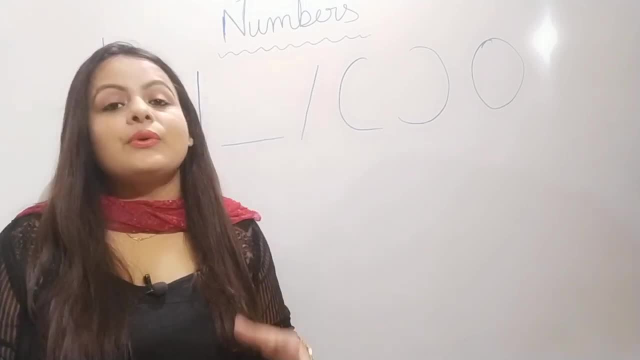 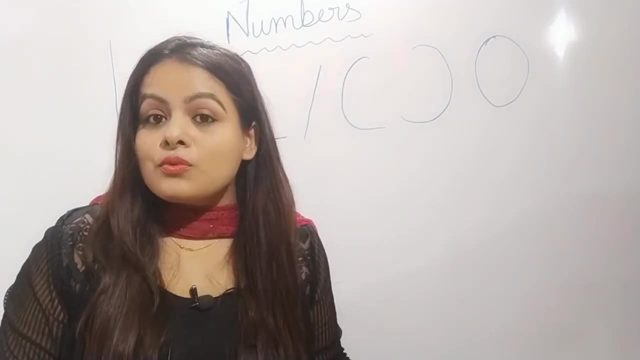 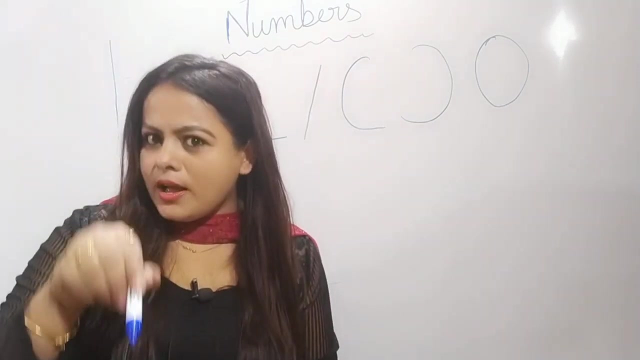 small circle. using these lines and curves, you can easily teach your little one to write and to remember the numbers. okay, so now let's start. so the first one is number one. okay, one stroke down, we have the one. one stroke down, we have the one. one stroke down, we have the one to make the number. 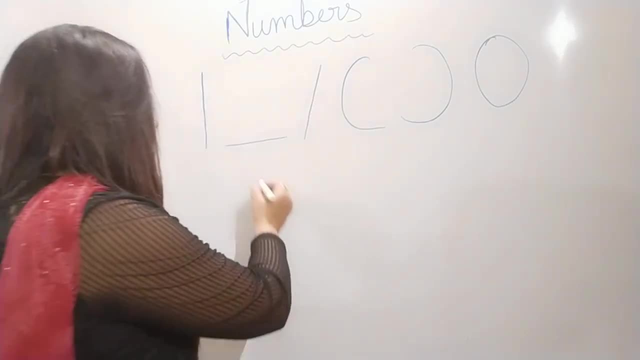 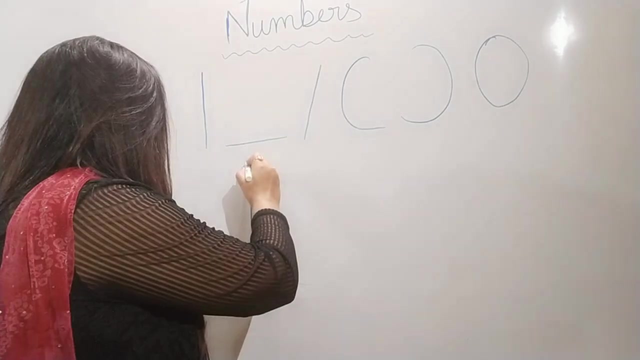 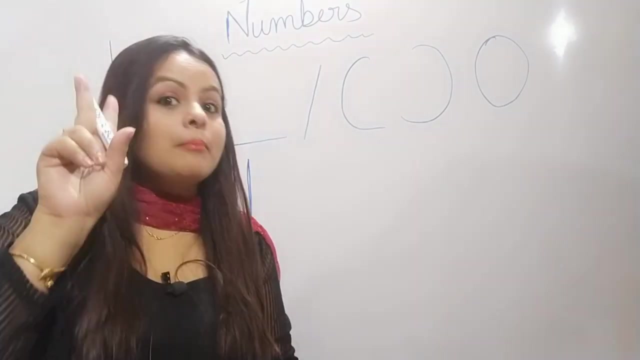 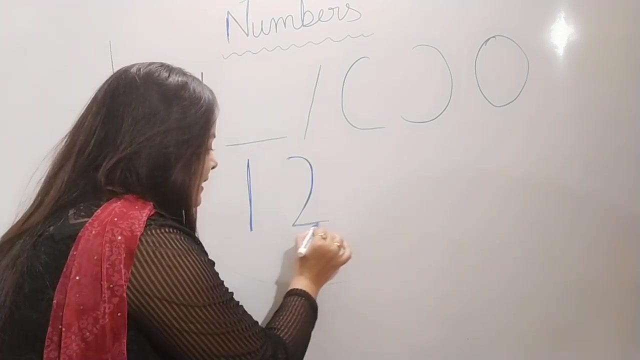 one. so now let's write the number one children down. we have the one one stroke down. we have the one one stroke down. we have the one to make the number one one. now. next number two: half a circle sleeping line. half a circle sleeping line, half a. 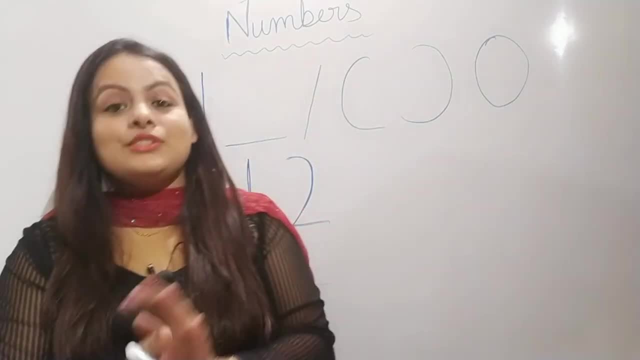 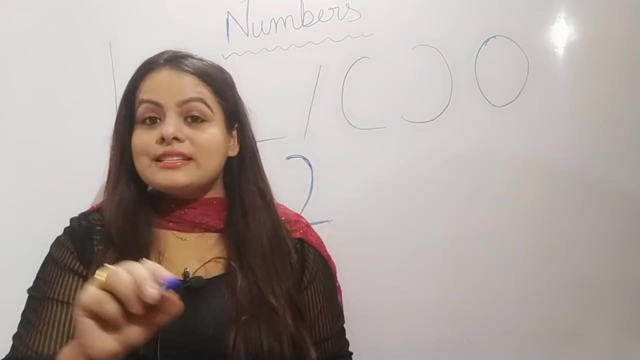 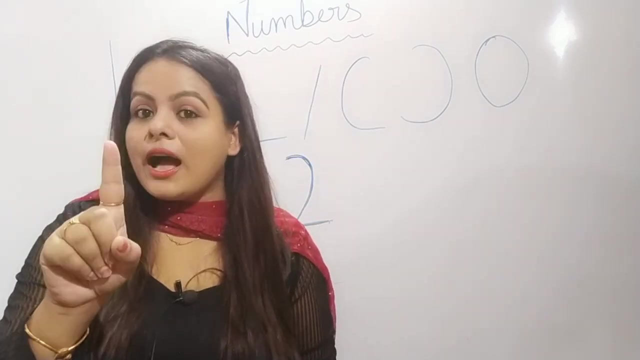 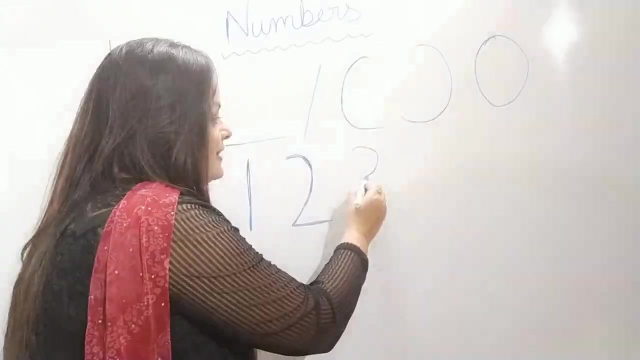 circle sleeping line to make the number two: half a circle sleeping line, half a circle sleeping line. half a circle, half a circle sleeping line to meet the number two: One, two, one, two. Now let's move towards number three: Half a circle, half a circle, half a circle, half. 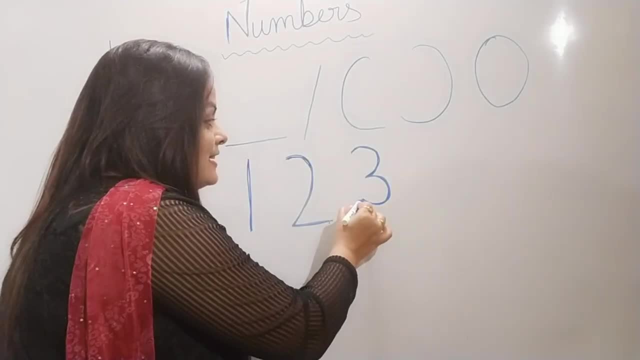 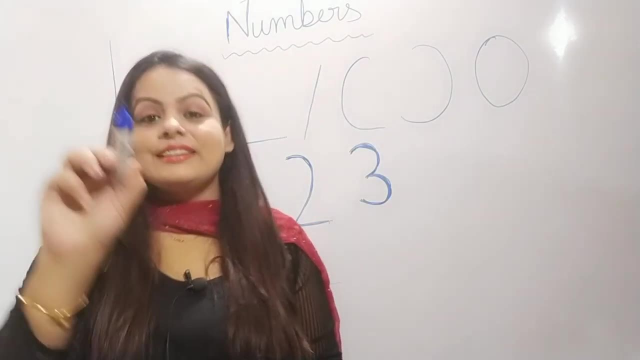 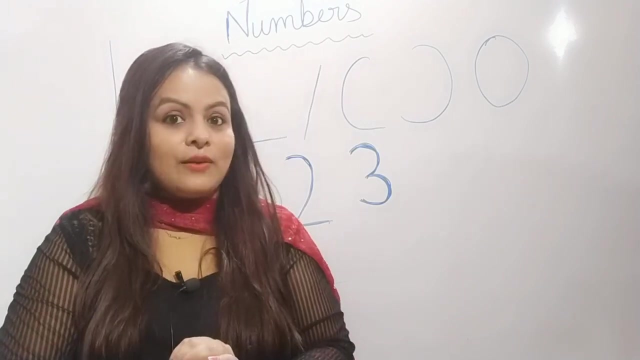 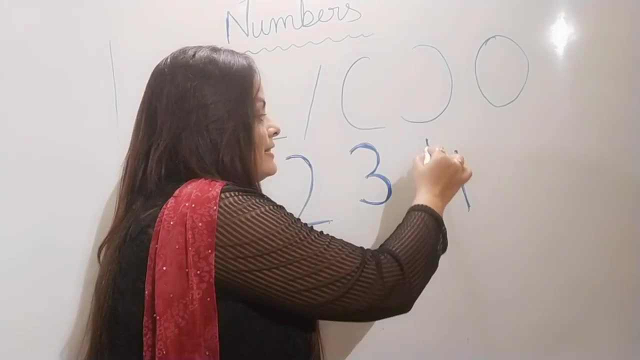 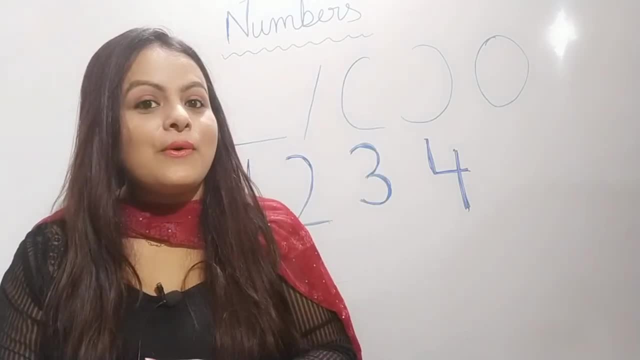 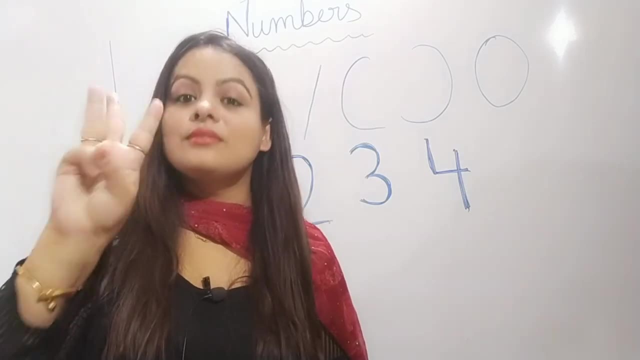 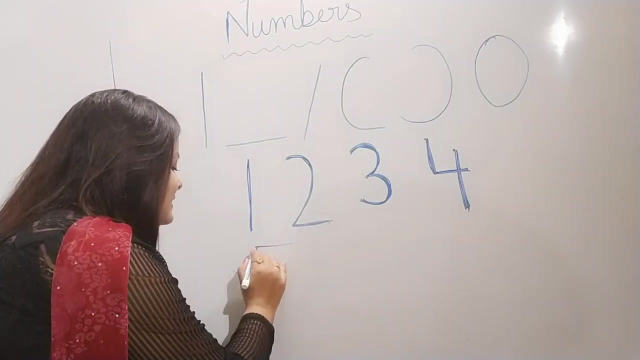 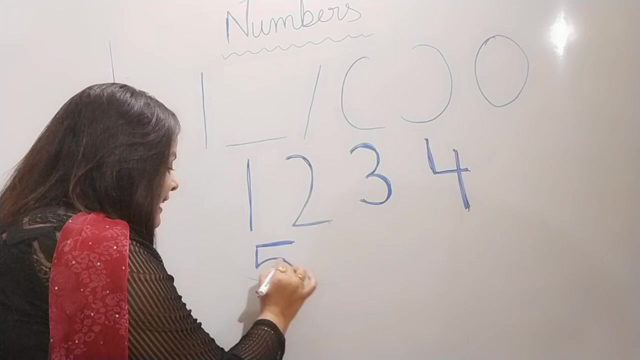 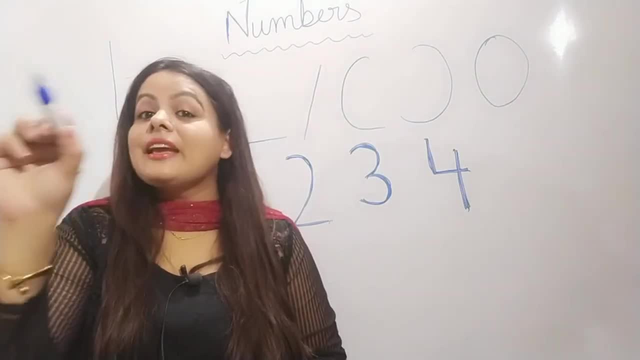 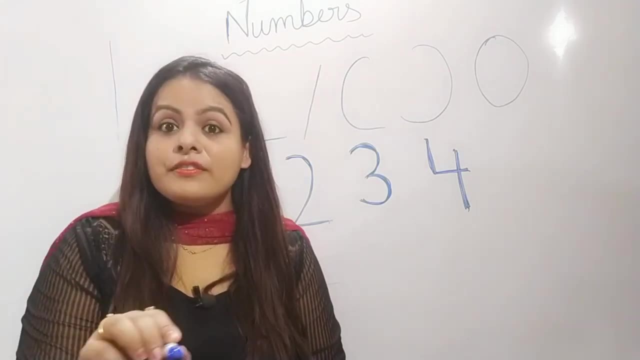 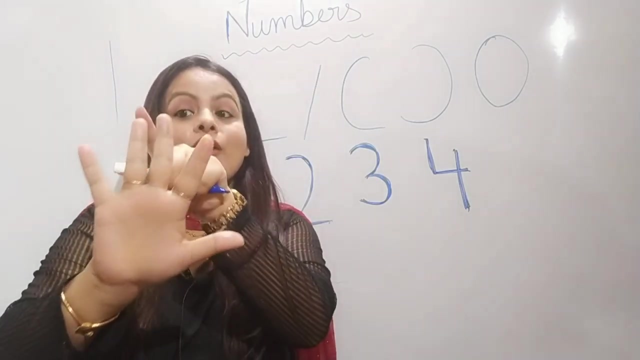 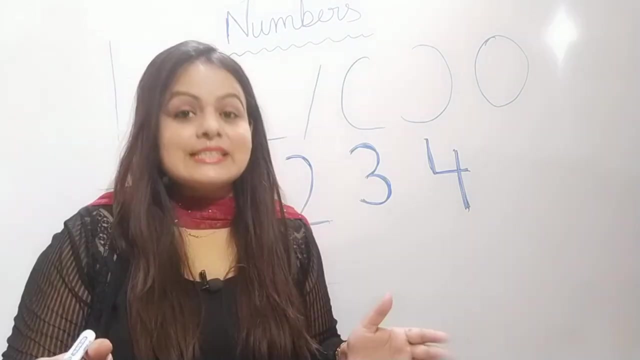 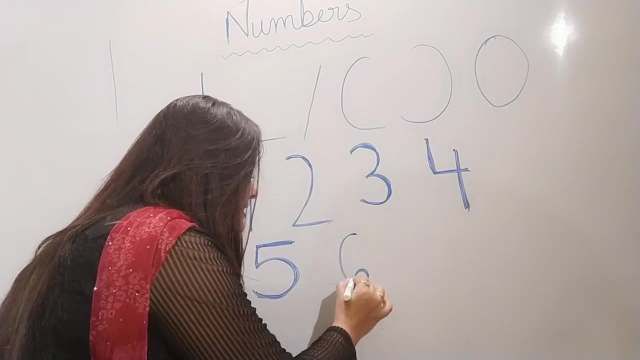 number five, sleeping standing half a circle. sleeping standing half a circle. sleeping standing half a circle. to make the number five: one, two, three, four, five. how many number 5.. Very good, Now next number 6.. Seek a van circle in Seek a van circle, in Seek a van. 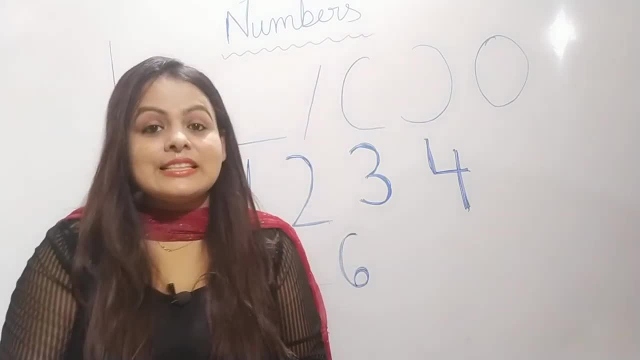 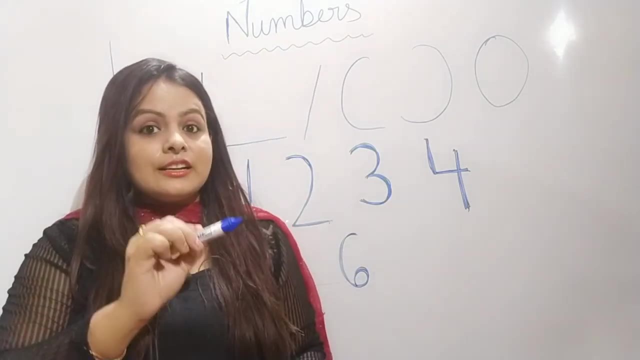 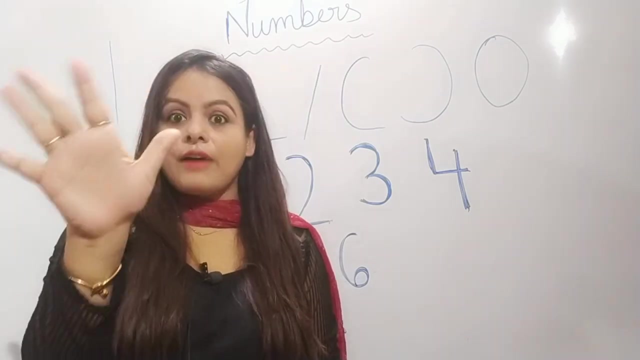 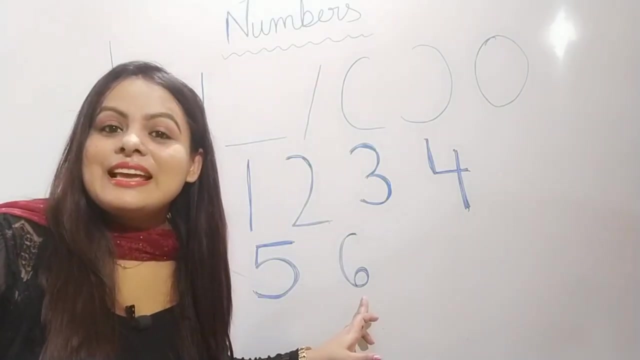 circle in to make the number 6.. Seek a van circle in, Seek a van circle in. Seek a van circle in to make the number six. one, two, three, four, five and six. how many six fingers? so here it is number six. now let's move towards the next number. 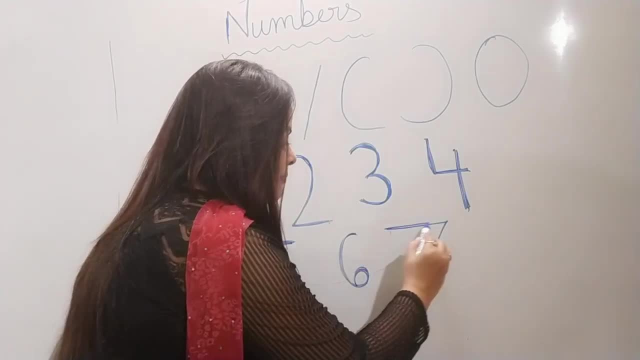 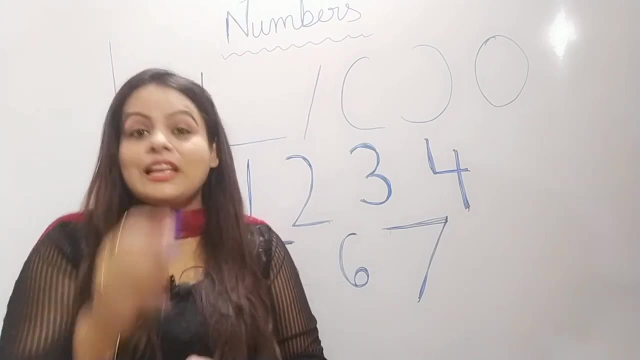 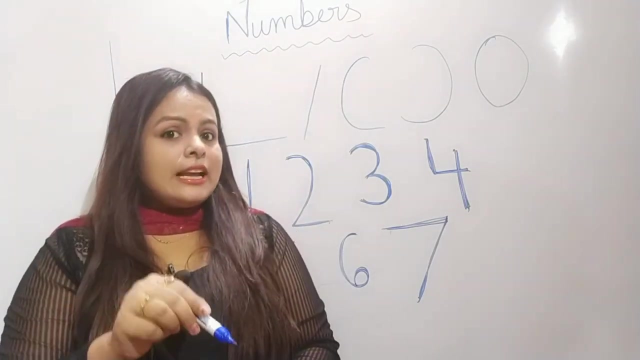 sleeping line and slanting line. sleeping line and slanting line. sleeping line and slanting line to make the number seven. sleeping line and slanting line. sleeping line and slanting line. sleeping line and slanting line to make the number seven. 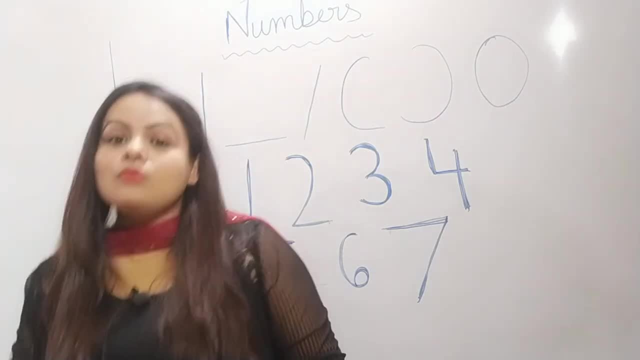 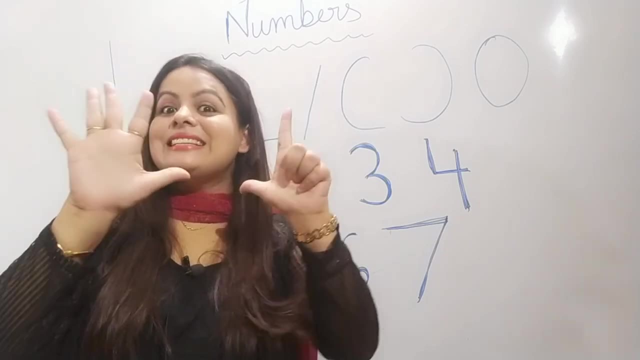 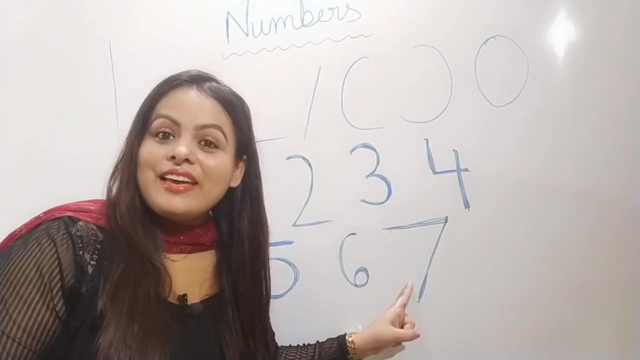 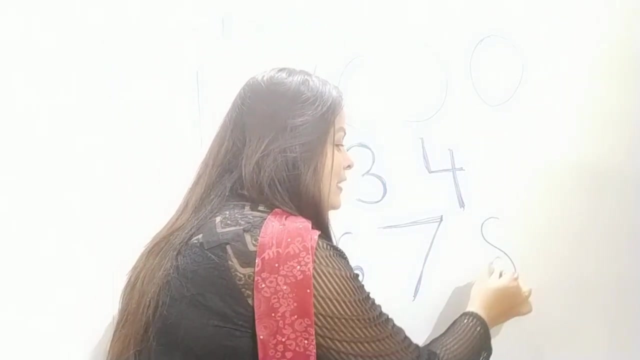 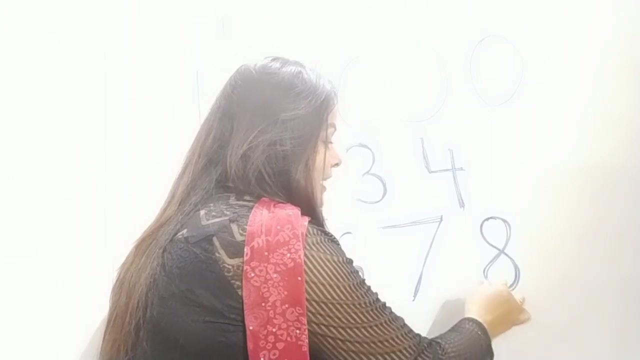 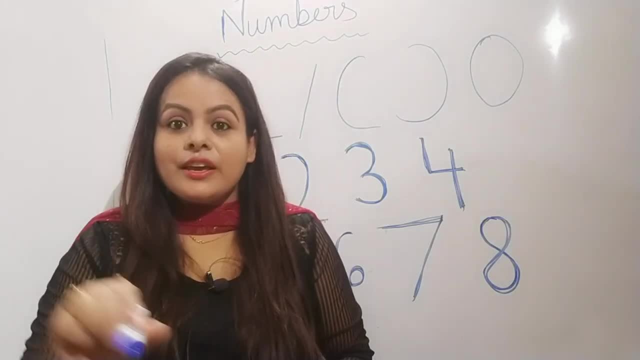 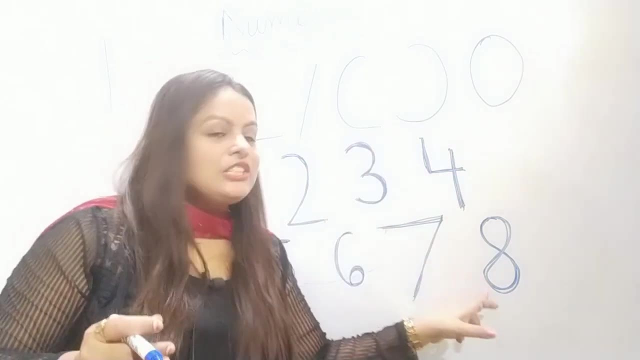 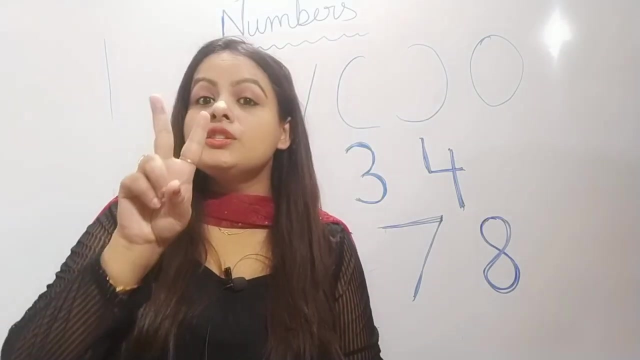 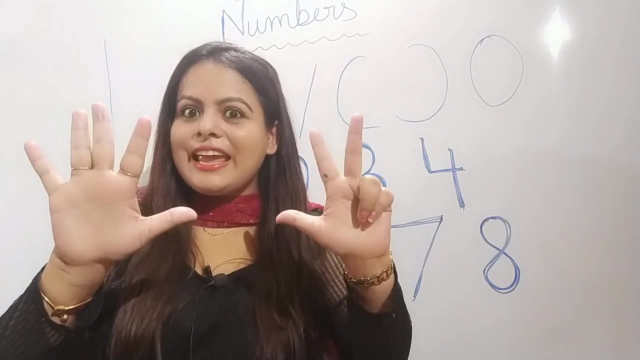 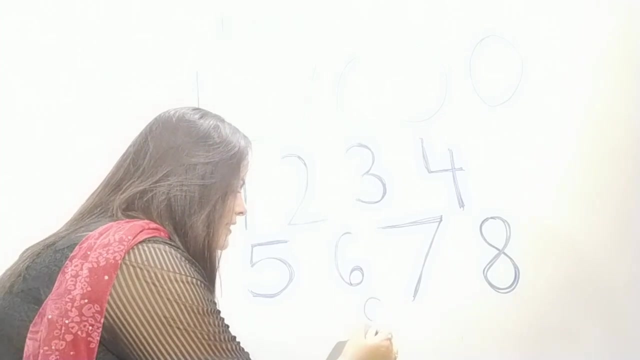 seek a way it goes up, seek a way it goes up, seek a way it goes up to make the number eight. which number number eight? okay, now let's count one, two, three, four, five, six, seven and eight. okay, now let's move towards the next number, number nine, smaller circle, standing line. 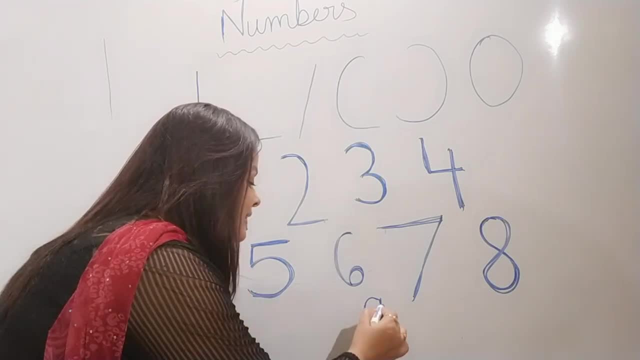 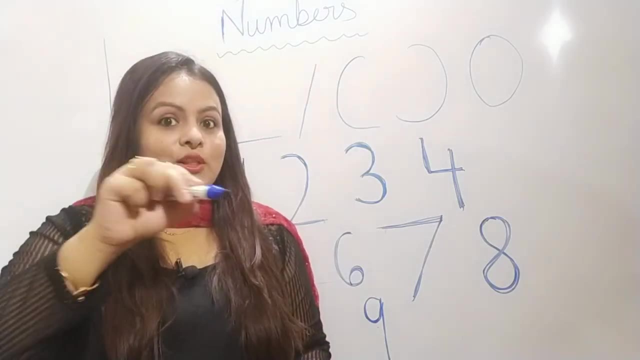 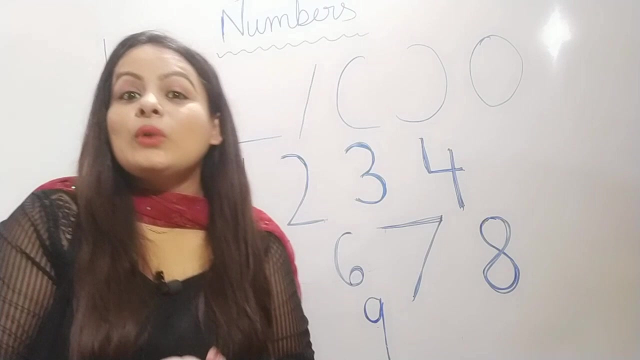 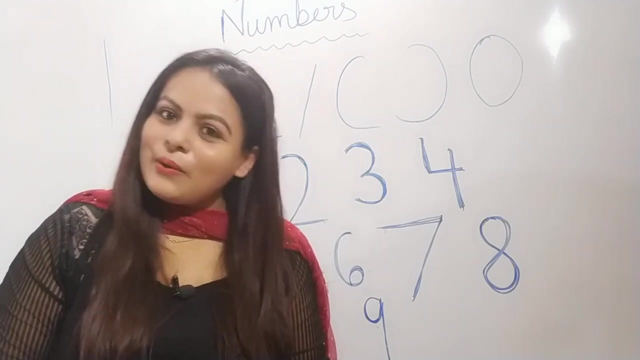 smaller circle standing line. smaller circle standing line to make the number nine. smaller circle standing line. smaller circle standing line. smaller circle standing line to make the number nine. which number number nine? very good, now, children, let's repeat the rhymes with action. okay, sing along with your mom one stroke down, we have the one. 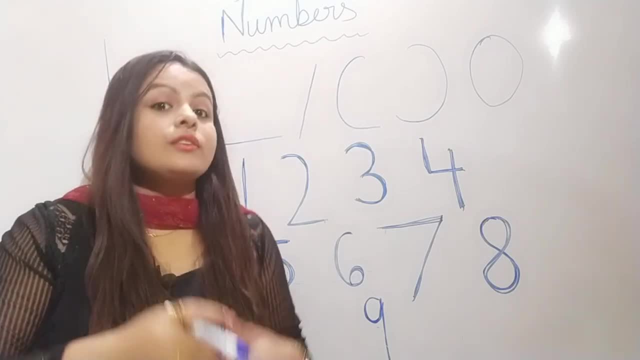 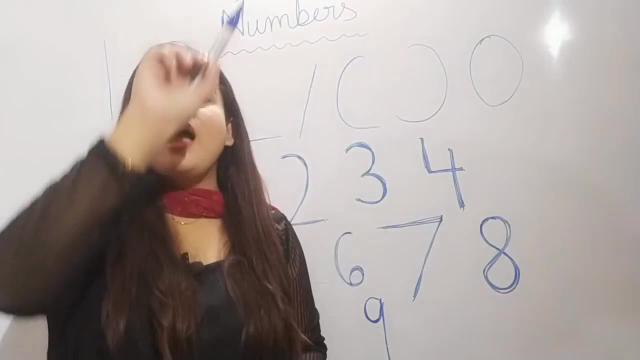 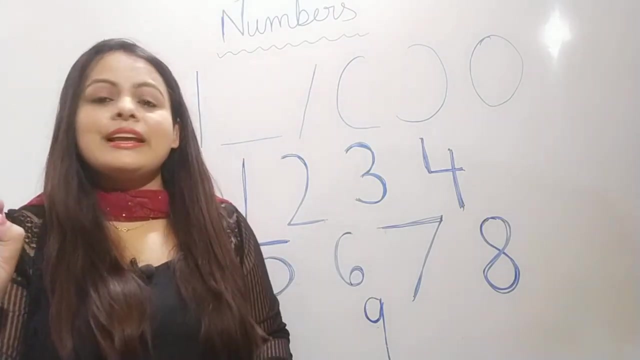 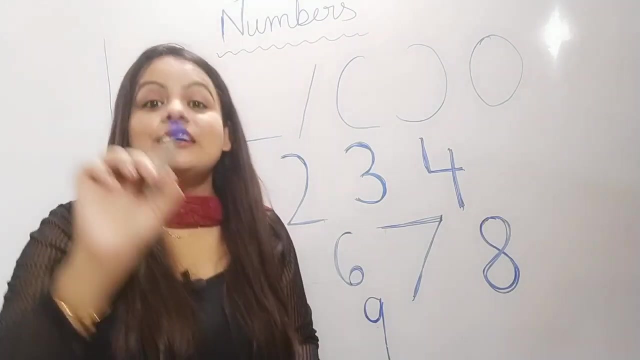 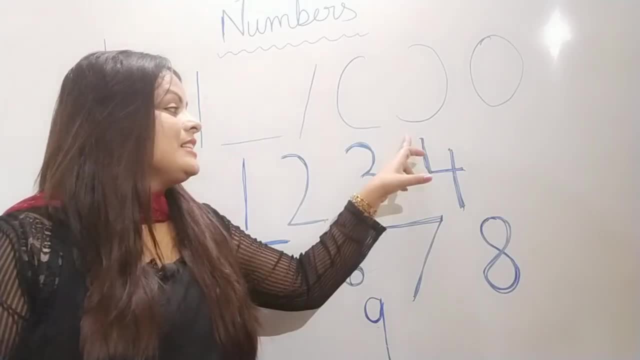 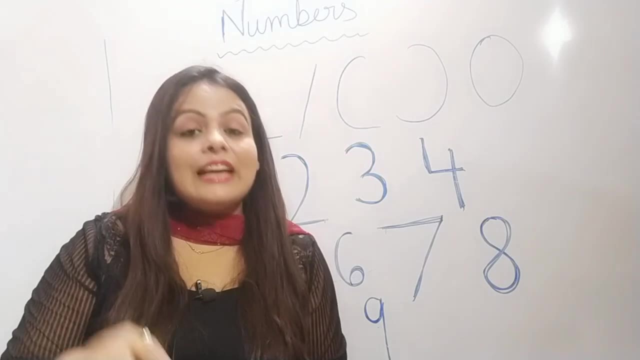 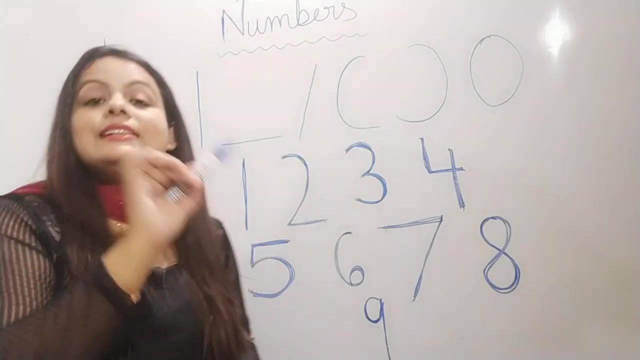 circle. the number three: Standing Slipping Standing line. Standing Slipping Standing line. Standing Slipping Standing line to make the number four. Very good, Sleeping, Standing half a circle. Sleeping Standing half a circle. Sleeping Standing half a circle to make: 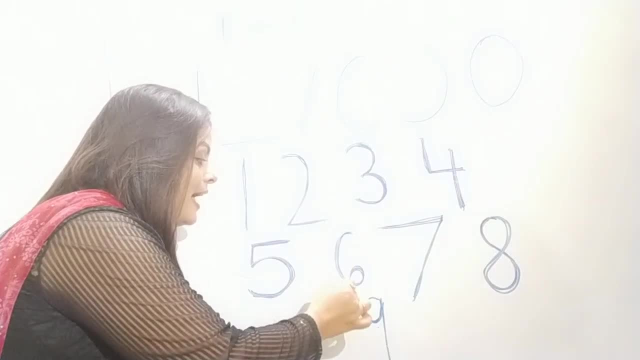 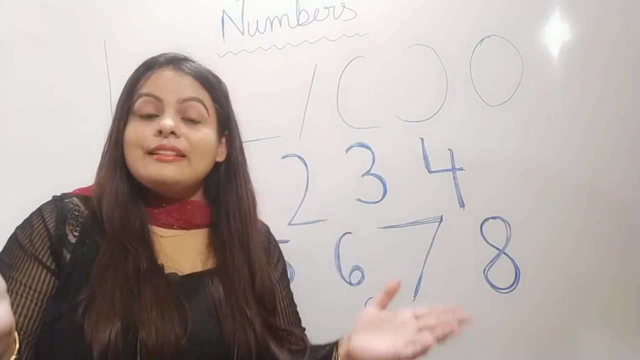 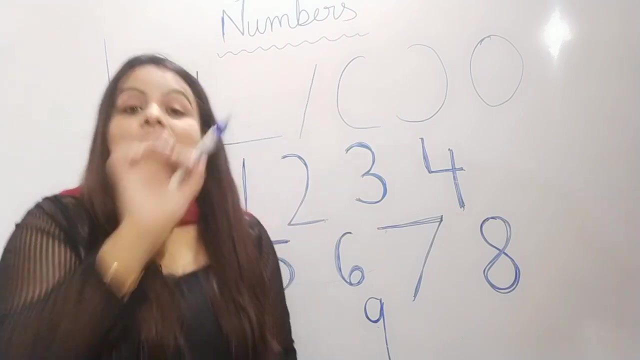 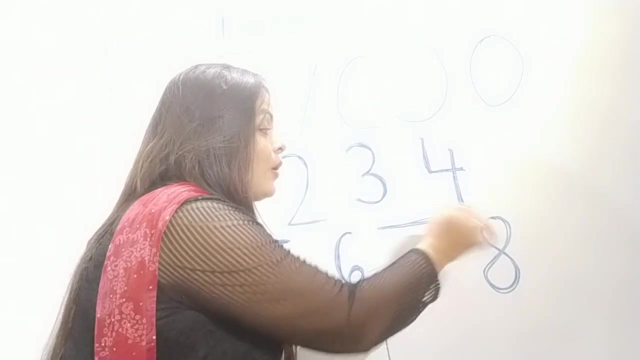 the number five: Seeker van circle in, seeker van circle in seeker van circle in. to make the number six: Sleeping line and slanting line, sleeping line and slanting line, sleeping line and slanting line. to make the number seven: Seeker van goes up, seeker van goes up, seeker van goes.